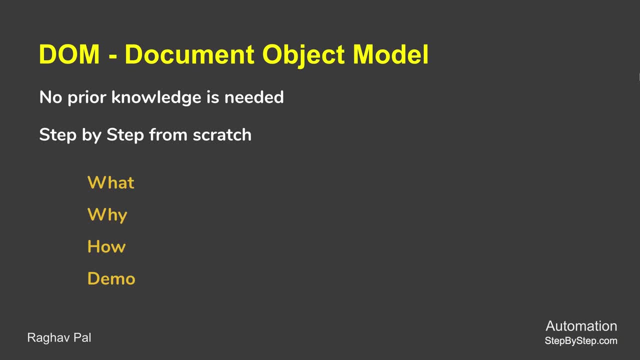 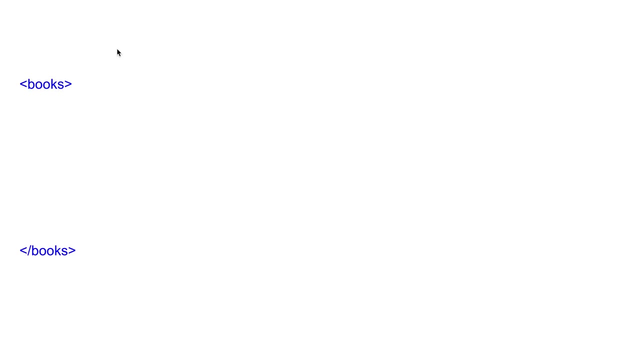 and start from scratch, and we are going to learn what is document object model, Why do we need it, How do we use it, And we are also going to see a very simple demo. So let's get started Here. I will start by creating a very simple XML. Here I have a books element, which 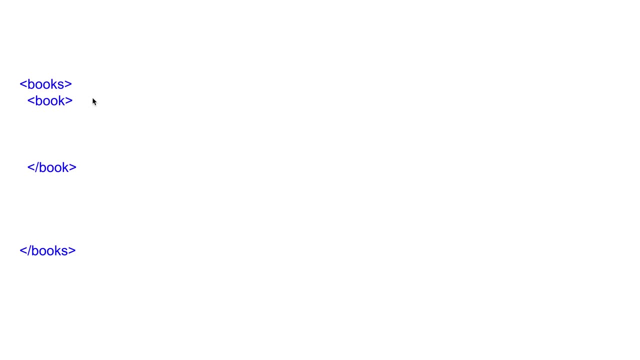 is the root element of this XML and under the books element we have book element. under book We have author, price and pub date, Then we have pub info element and under this we have publisher and state. So here books is the root element and then we have book and 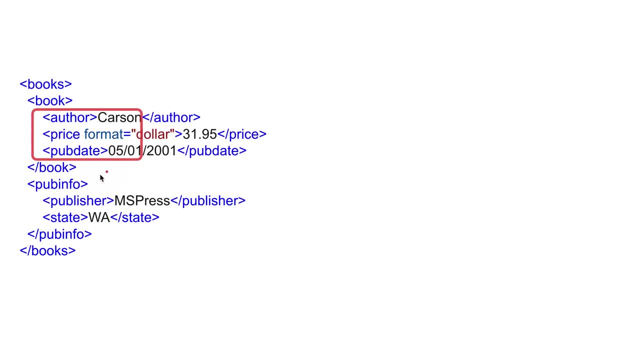 pub info as its child element. Under book, We have these elements and then under pub info, we have publisher and state. Now, if I have to represent this XML as a tree structure, I will start with the root element, that is, books. Under books we have book and pub info. Under book element, we have author price and 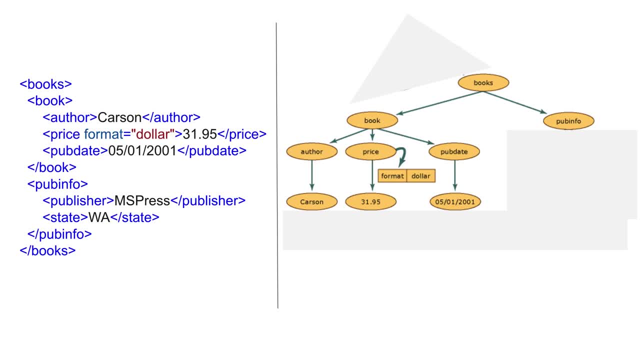 pub date, And these are the values for these elements. Then, under pub info, we have publisher and state, And these are the values. These are the values for these elements. Now, this is a very simple tree structure, or a tree view of this XML, And we have converted our XML as a tree view And this is exactly. 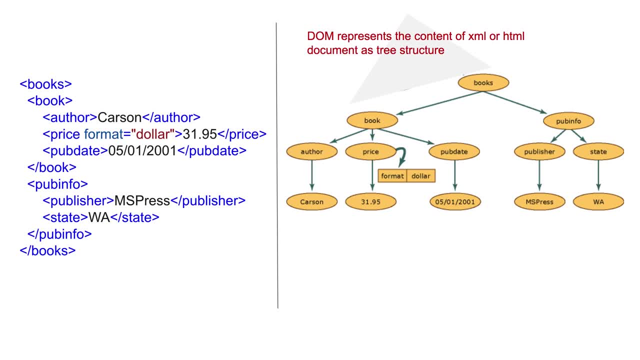 what DOM does. DOM represents the content of a XML or HTML document as a tree structure, and DOM is a programming interface or an API, And this API can be used with any programming language. Most It is used with JavaScript and using DOM, we can easily read, access and update the contents. 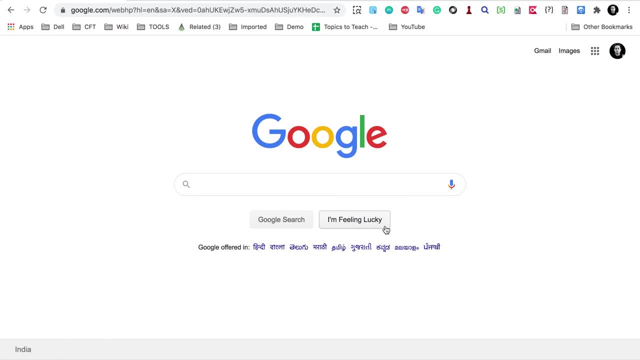 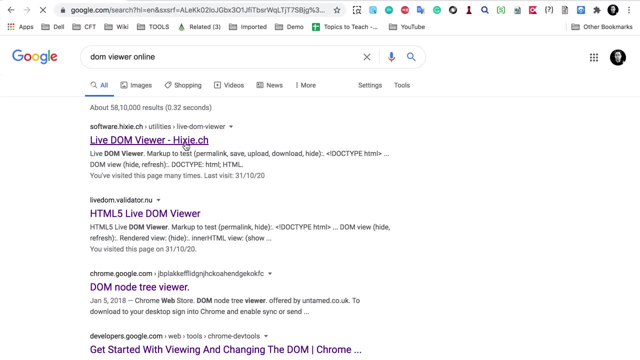 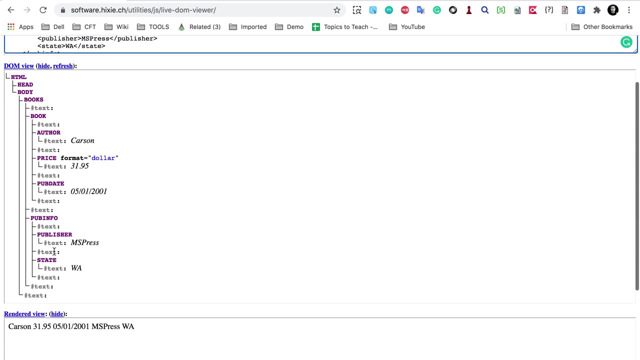 of the document. Let me show you some example. I will go to Google and search for DOM viewer online And here I will go to this live DOM viewer And if I give my XML here, you can see it has converted it into a tree structure. So this is what DOM does, And DOM does this. 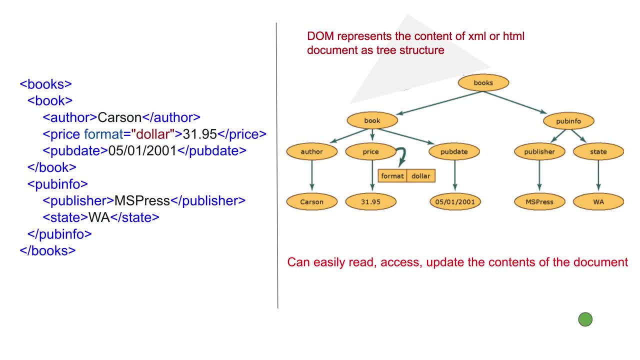 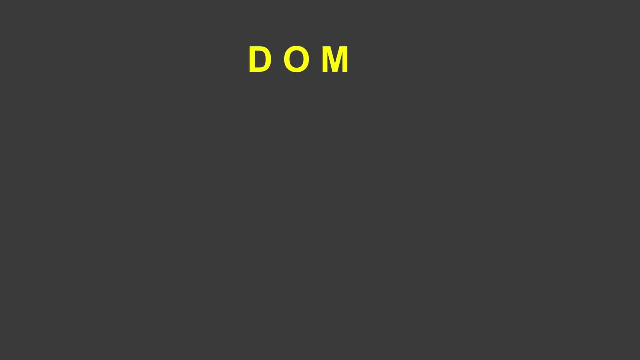 conversion into a tree structure internally in the memory and then, using the program of the language that we are using, We can then use it to access and update the contents. So to explain in very, very simple words: DOM stands for document object model, where document is the file, like a HTML file or an XML file, Object are the tags and the elements of that. 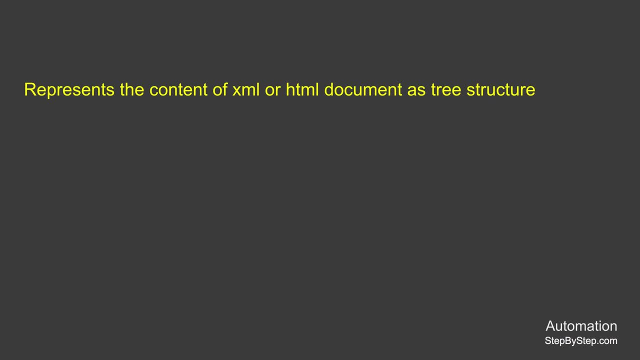 file and model is the layout or structure. So The object model or DOM represents the content of XML or HTML documents as tree structure. It can be used to easily read, access and update the contents and is a programming interface or an API, And it represents the document as a tree structure internally in the memory. 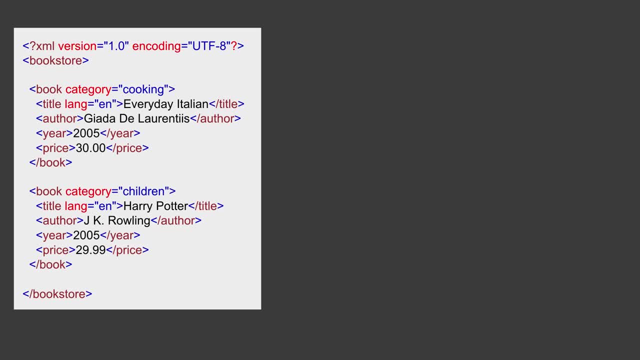 and can be used with programming languages like JavaScript Here. If you see, this is a simple XML where we have bookstore as the root element And then we have element for book. We have title, author, year, price. Now DOM can convert this into a tree structure. 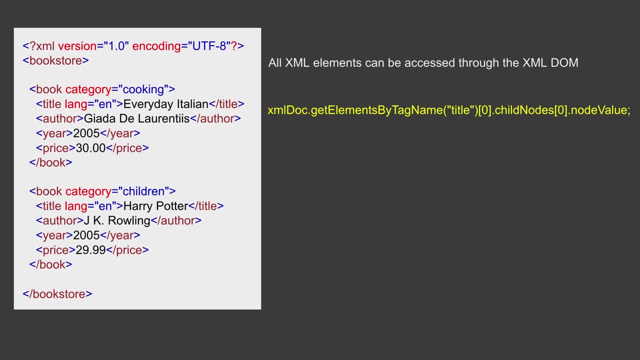 And then by using the DOM functions like get elements by tag name, we can access the elements. So here you can see, we have used a script, dot get elements by tag name, title and its child node, And using this we can retrieve the text value of the first title. Let me show. 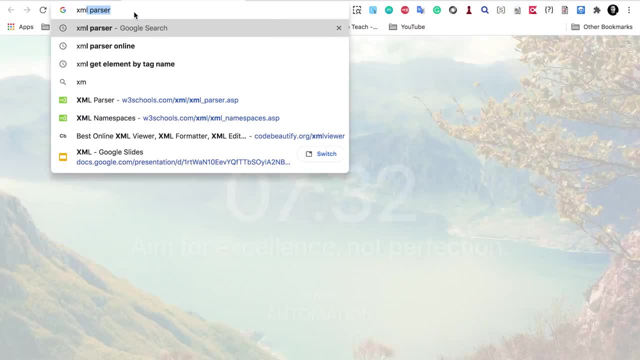 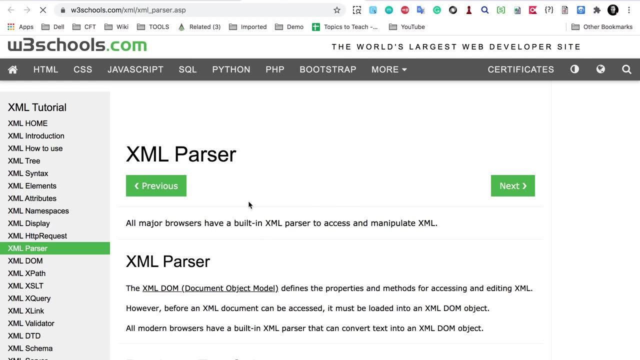 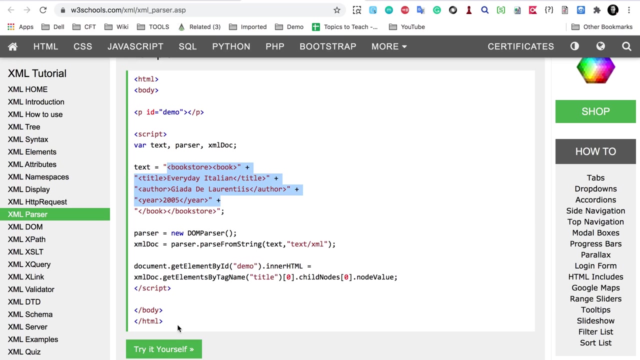 you this in action. I will go to Google and search for XML parser And here I will go to W3 schools And this is the example I have taken from here, So you can see this is the same example, Bookstore book And this is the title, author, etc. I will 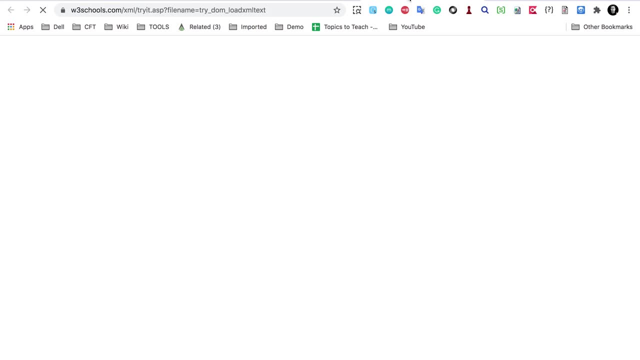 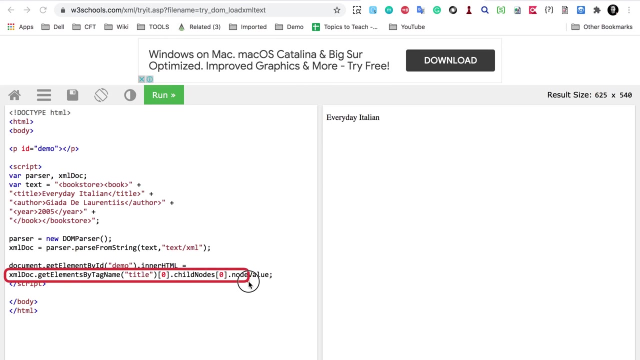 click on, Try it yourself So it will open an editor And here you can see. this is our script: get element by tag name, title zero, child node zero, And in the result we are getting everyday Italian, Which is coming from here. So it has accessed this element using DOM And if I just change, 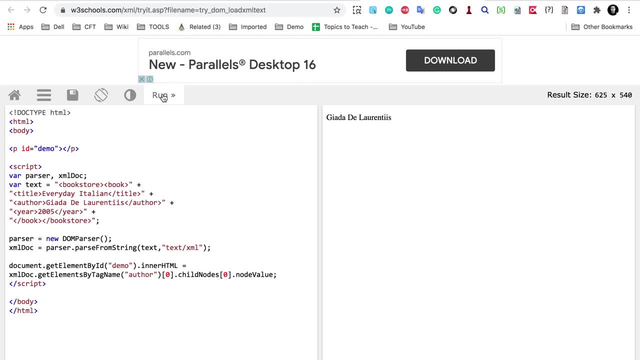 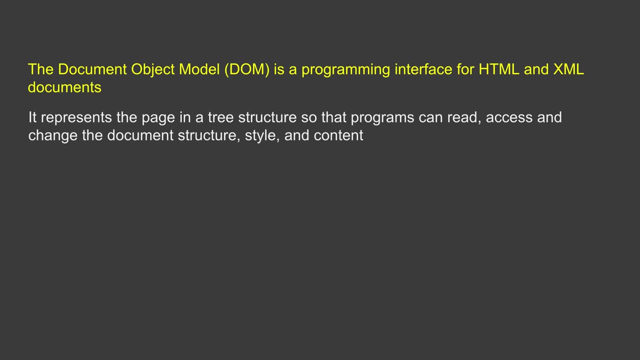 this title to, let us say author, and I say run. you can now see it is accessing the author here and this is here, And then we can also modify it if we want to. So here we now know. DOM is a programming interface for HTML and XML. It can be used to represent the page as: